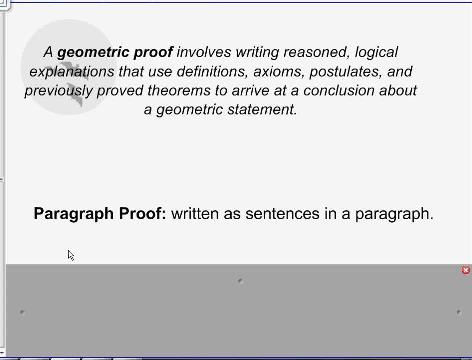 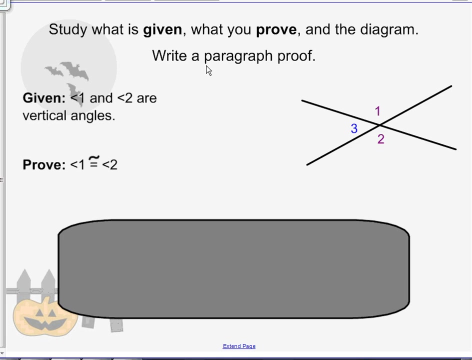 A paragraph. proof is written as sentences in a paragraph. So as we go into geometry a little bit more, you're going to notice there are two other types of proofs that are more mathematical looking. This is going to look more like an actual just paragraph written with a bunch of math terms in it. Okay, so what we're going to do right now is we are actually going to go over what a proof looks like. Okay, so your first step is to 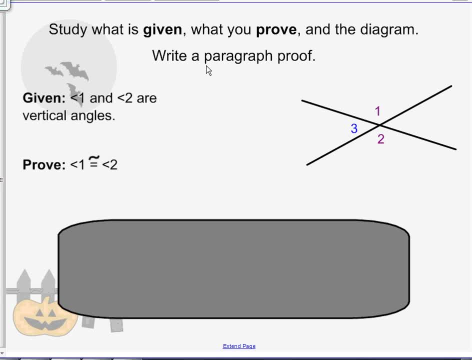 is you're going to study what is given, what you have to prove and the diagram that you're given Okay. so in this case, the diagram would be this And you have to write a paragraph proof about this. So in every proof, you're going to get a picture or a diagram. you're going to get something that is given Okay, and then you're also going to give something that you need to prove to be correct, And you're going to need to do that in a series of different ways. One of the most important things about proof is that you're going to need to do that in a series of different ways. 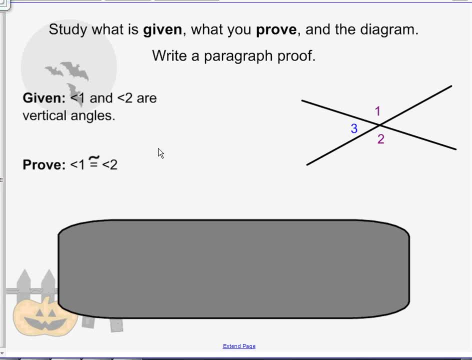 One of the most important proofs is: you cannot assume that something is already stated or that it should just be implied. You need to be very specific. Okay, so just to break it down, So this is what you know to be true And this is what you show. Okay, so if you take, if you take your diagram and you and you start to think about it, All right, so 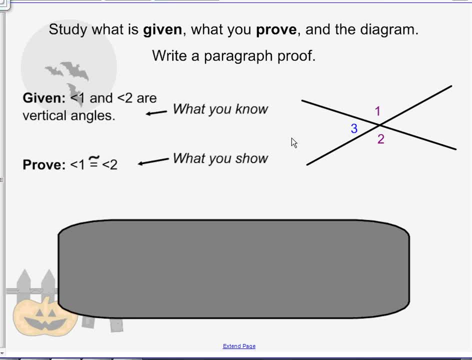 we can go through and we can actually write a paragraph using some of the theorems you learned yesterday. We learned a lot about the different vertical theorem, vertical angle theorems- excuse me- that you can use in order to solve this right away. you know, okay, we're working with vertical angles, Okay, And the vertical angles are angle one and angle two. Okay, Now, knowing the definition of 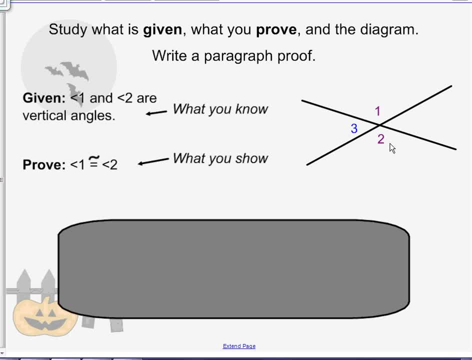 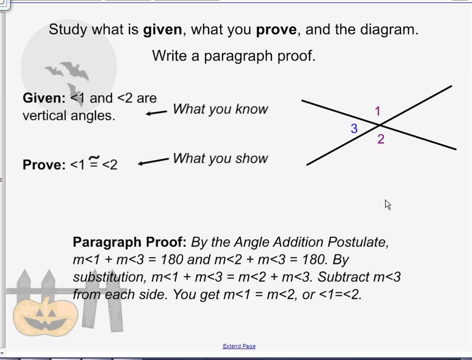 vertical angles, we could probably safely assume that angle one is congruent to angle two, But we need to prove that correct. Okay, And it's going to seem very roundabout, but I promise it'll make more sense as we go. Okay, So the first thing is I'm just going to show you what the answer to this particular paragraph proof would look like. So, by the angle addition postulate, okay, which we learned. 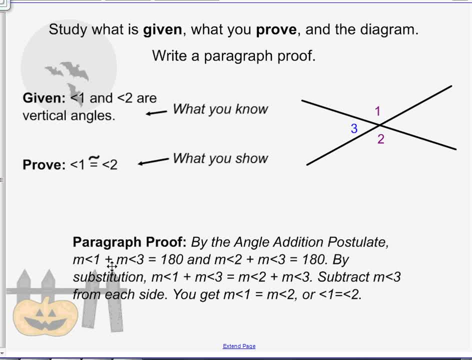 about. we can say that measurement of angle one plus the measurement of angle three equals 180.. So we're talking about this angle and this angle equal 180 degrees, And we can see that because this is a straight line And they are collinear angles. Okay, We also know that angle two 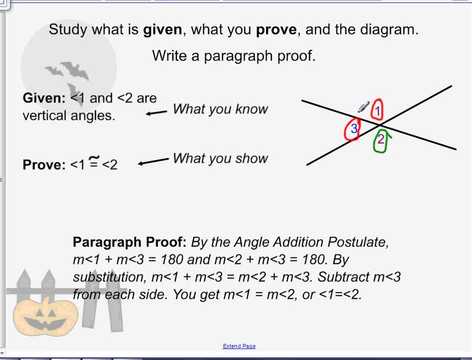 and angle three are also 180 degrees. So by substitution, okay, we can actually create this equation right here. So we know that measurement of angle one plus the measurement of angle three- which is what was up here, Okay- And the measurement of angle two plus the measurement of angle three, both equal 180 degrees. So they actually equal themselves Now by subtracting measurement of angle three out. 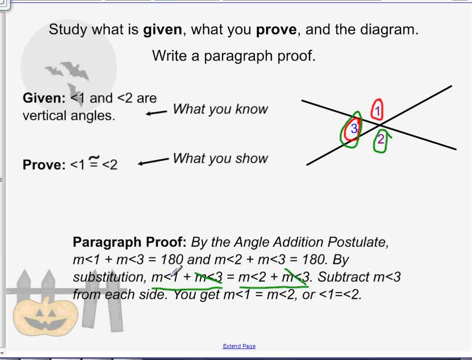 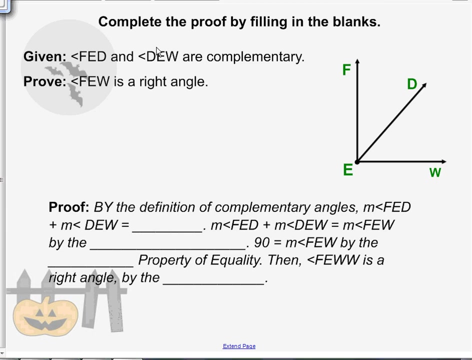 of both of these, we actually get that measurement of angle one equals the measurement of angle two, or that angle one is congruent to angle two. All right, I know it seems very confusing. All right, We're going to do one more example and then it should make more sense. So here's our example: We have complete the proof by filling in the blanks And we're given that angle FED. 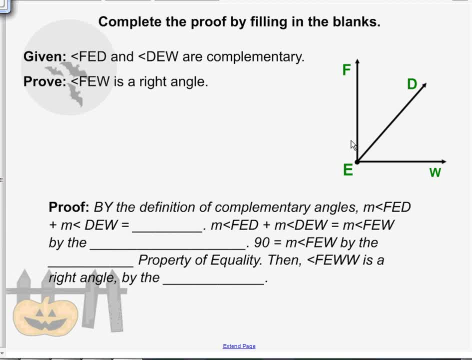 and DEW are complementary And we want to prove that those two are right angles. Now we're going to just fill in to the proof that is given here. So it says, by the definition of complementary angles, the measurement of FED and the measurement of angle DEW is going to equal because they're complementary.